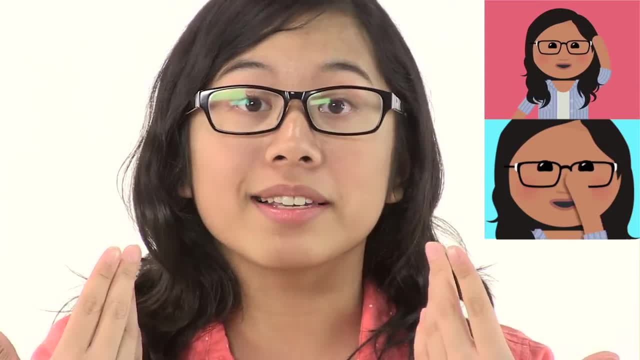 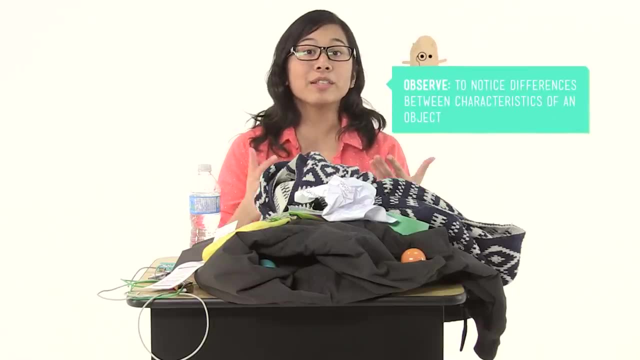 my characteristics include having black hair, wearing glasses, having some wicked awesome nerd cred, and well, you get the idea. Properties of matter are also things that we can observe. This means that they have differences that are big enough to notice. For instance, I'm currently 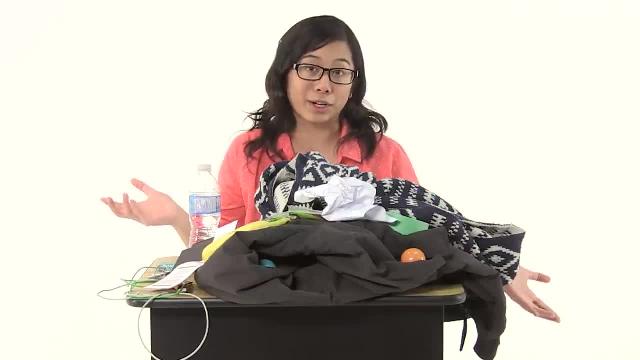 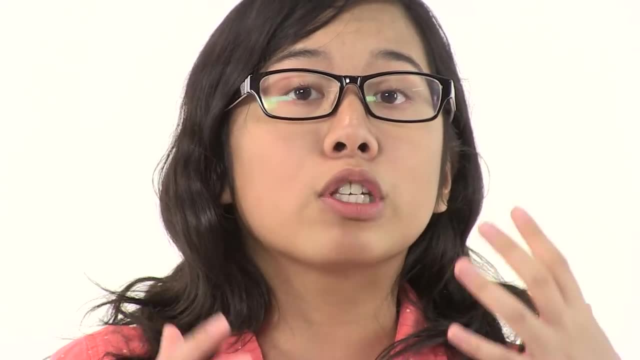 observing that my desk is messier than it was five seconds ago. And to round it out, properties of matter are also able to be measured. That is, we can compare objects to each other, But instead of just looking at them and getting a general idea of how they compare, we measure them by using tools. 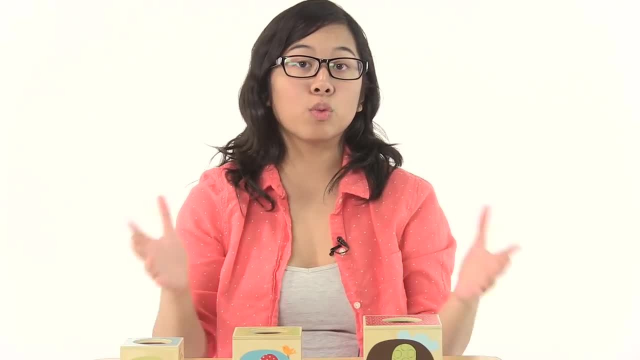 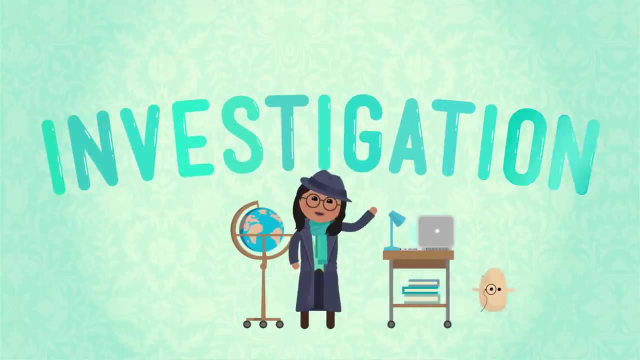 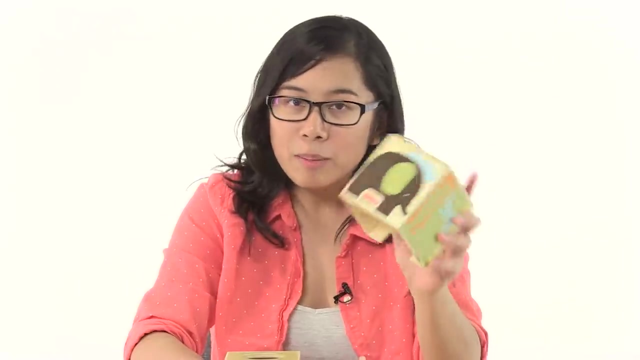 Now let's put all of these ideas to work by demonstrating how we can find a few basic properties of a simple object. Let me grab my measuring tape, Hmm, Okay, okay, look, I know I was just talking about how fun it was to play with blocks, but let 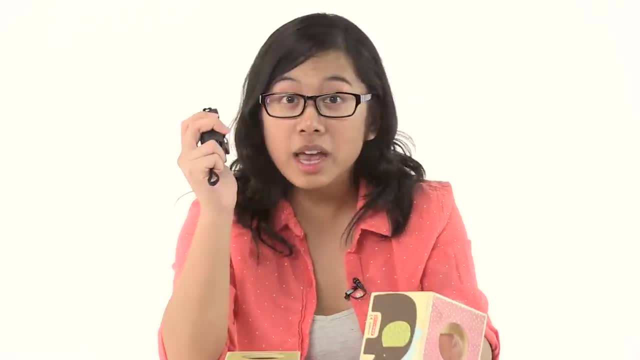 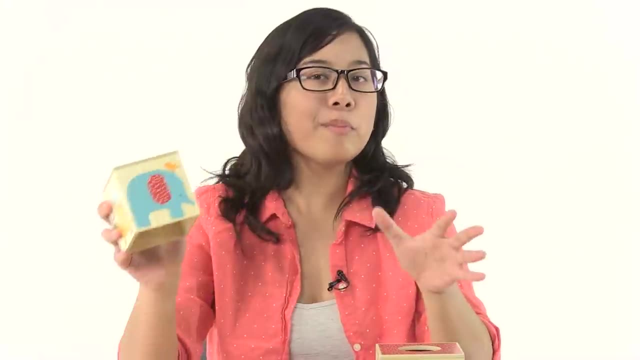 me be clear: I am not playing with these blocks. This is science, people. Now let's start with a couple of questions. One: what properties does this block have? Well, there are some properties, but we can't really measure or describe them with numbers, like this block's color or what it's made. 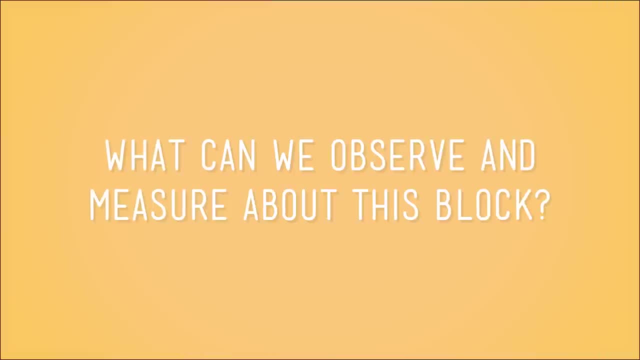 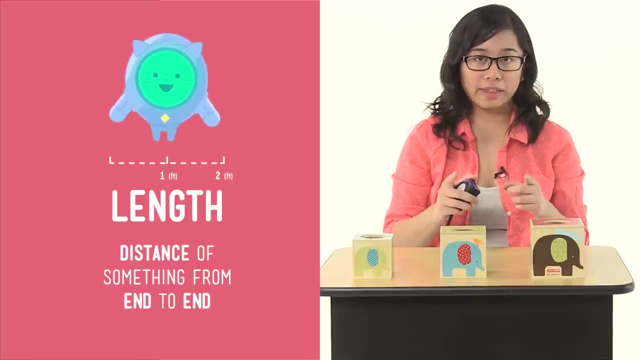 of, or even the fact that it holds its shape, which makes it a solid. So a better question to ask might be: what can we observe and measure about this block? Let's start with the big one here: length. Length is just the distance of something from end to end, And this block's length is eight and a half. 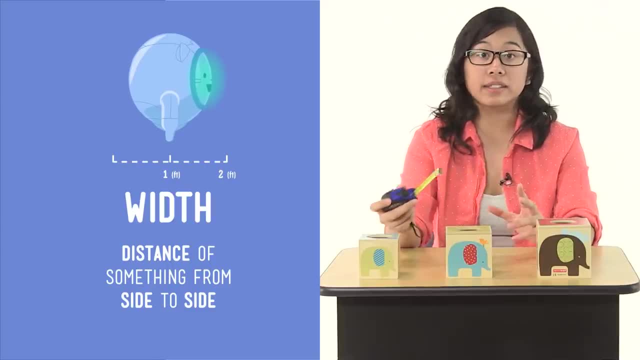 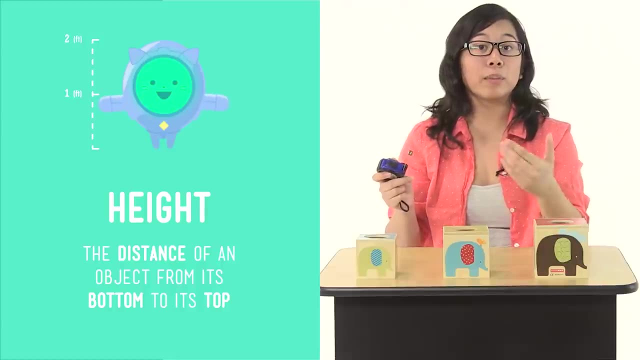 centimeters. Width, meanwhile, is the distance of something from side to side, and its width is eight and a half centimeters Height. That's an easy one. It's the distance of an object from its bottom to its top, not to mention a major factor in being. 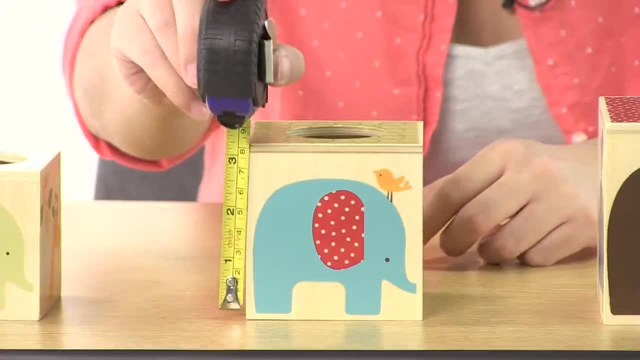 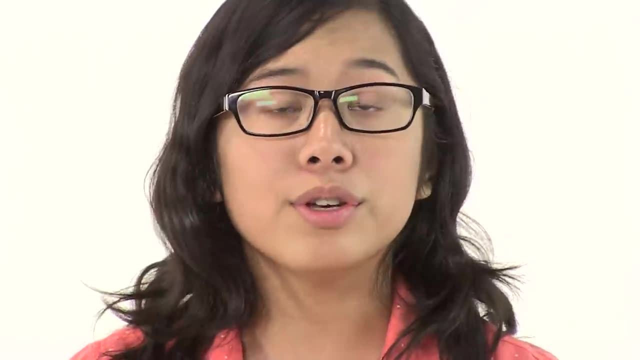 able to play basketball successfully, And the height of this block is nine centimeters. So length, width and height are some of the most commonly used properties, but there are a lot of others too. For instance, our block is also an object shaped like a box that takes up space. 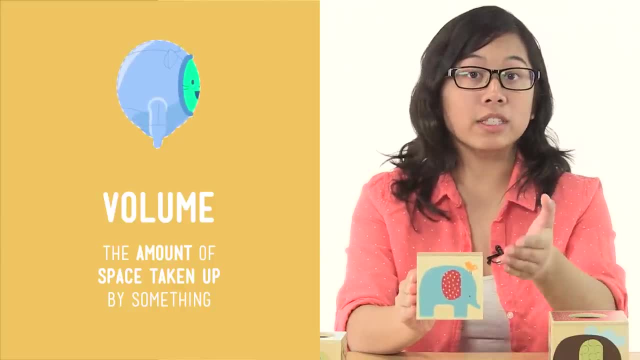 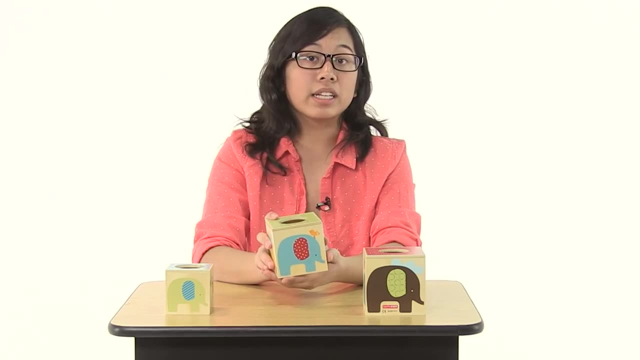 That is, it fills up the space it's in. We call that space the block's volume. We can measure the volume of this block using math, based on the measurements that I just made, But we can also get an idea of its volume by making other observations. Like the medium block easily fits into the bigger